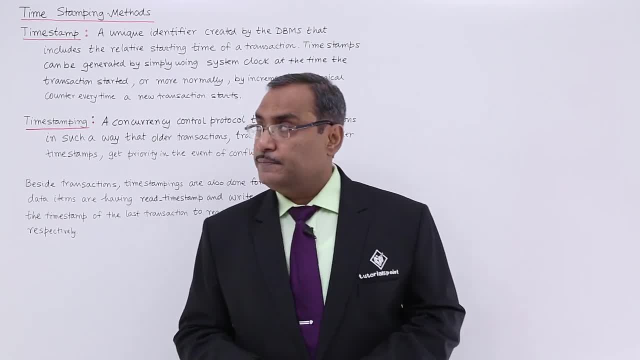 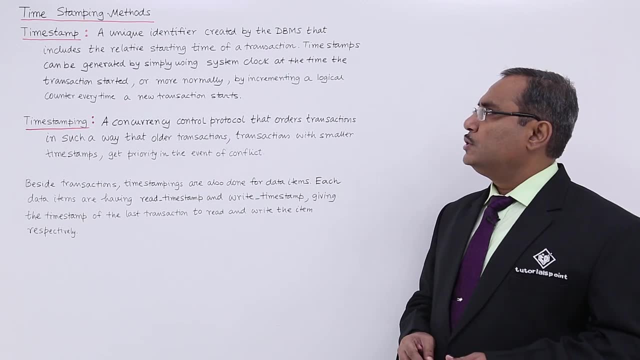 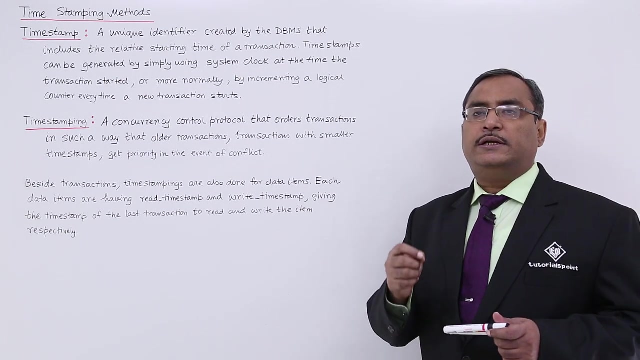 time stamping. So let us go for the text at first. So time stamp? a unique identifier created by the DBMS that includes the relative starting time of a transaction. Time stamps can be generated by simply using system clock, as we have discussed that each and every transaction when its origination. 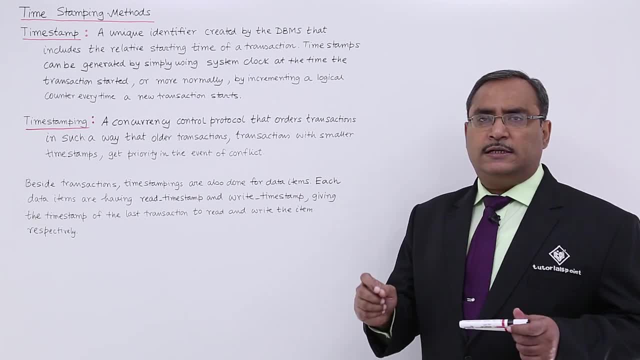 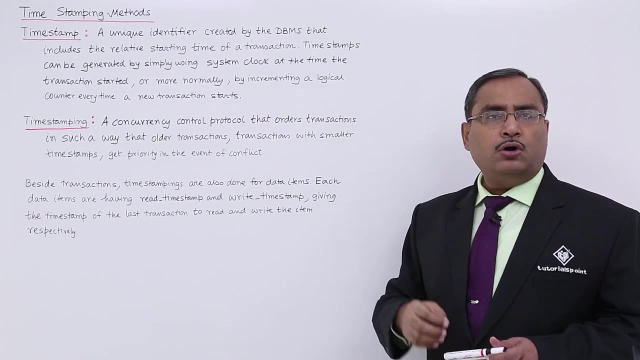 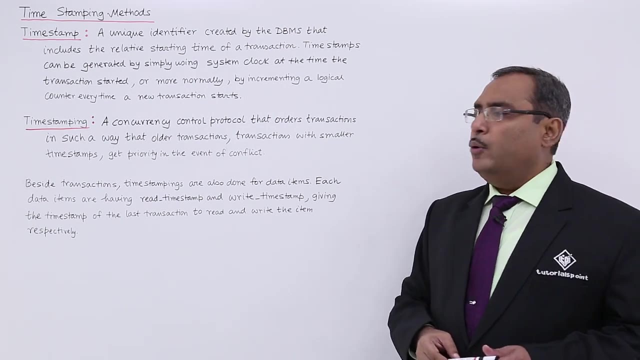 time, along with the minutes, along with the seconds, may be with the fraction of the second. So that will be the system: clock at the time the transaction started or originated, or, more normally, by incrementing a logical counter every time when a new transaction will be. 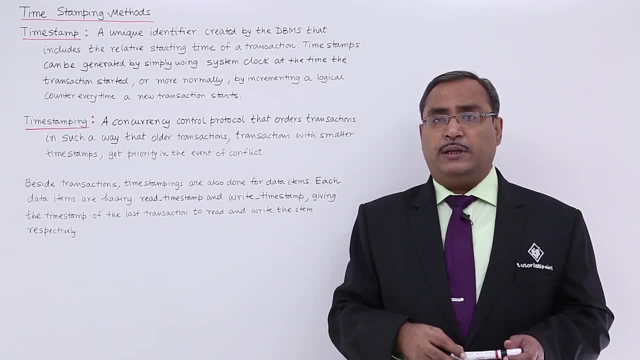 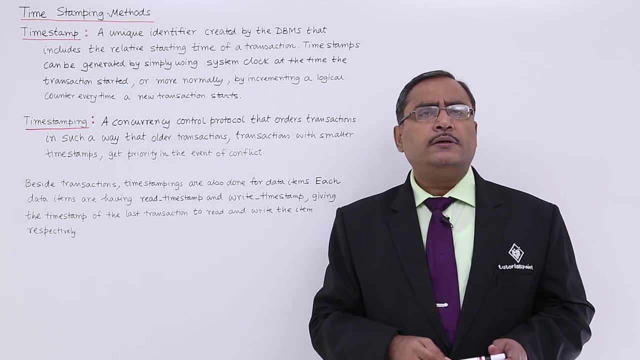 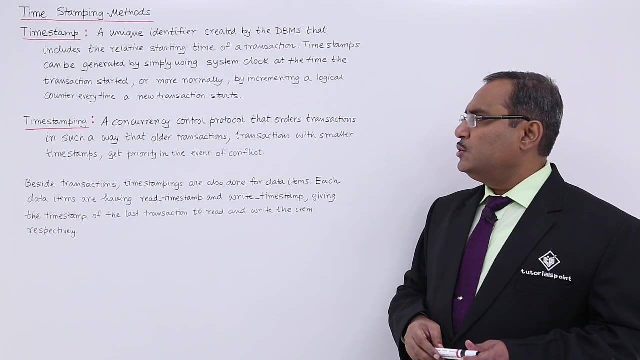 originated. So these are the very common methods. Now let us discuss the term time stamping: A concurrency control protocol that orders transactions in such a way that older transactions, transactions with the smaller time stamp, get priority in the event of conflict. You see how to detect that this transaction is older. 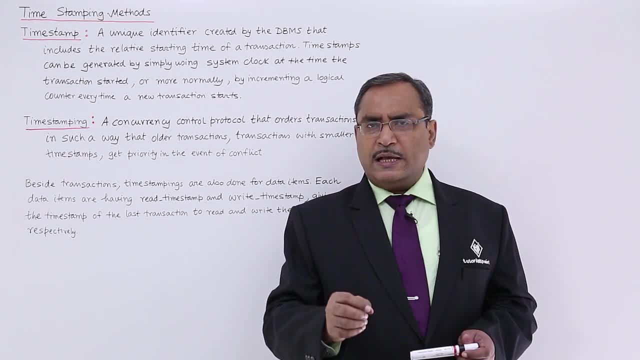 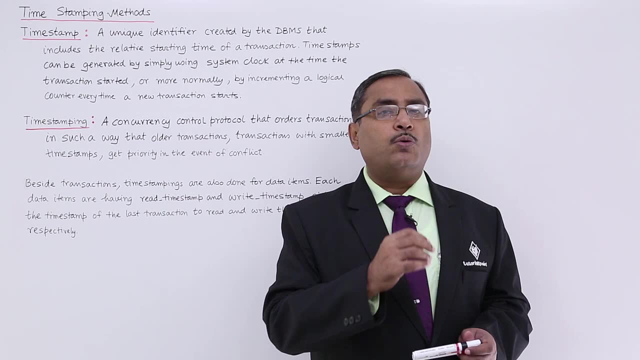 and this transaction is younger. When it comes to insider transactions, you can see that the data item on this database base appears a little normal. If the timestamp has been done using system clock, the system clock value is lesser for a certain timestamp, ie that is the older one. 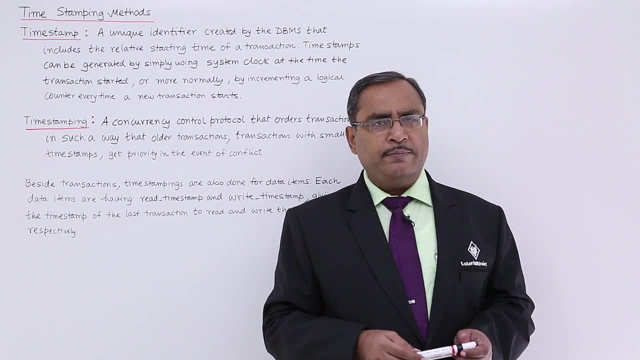 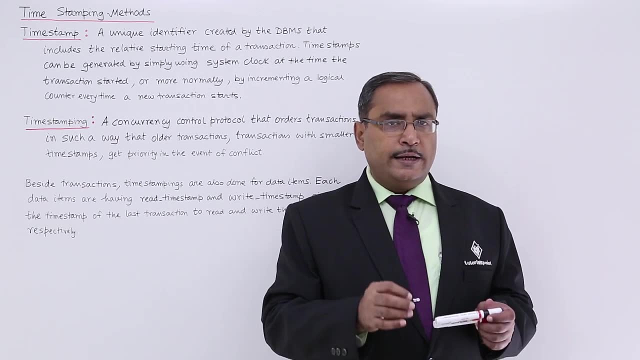 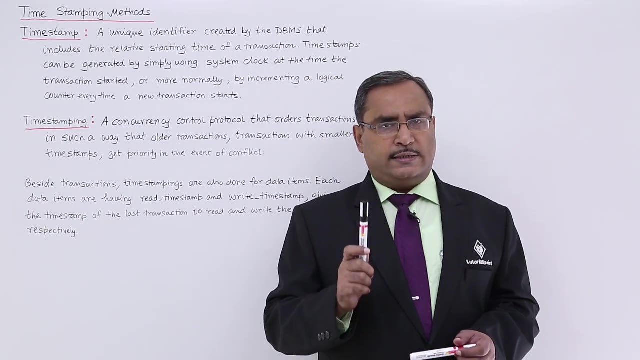 If you go for logical counter incrementing each and every time, then also the lower counter value against the particular transaction will indicate that it is the older one. Whenever there will be some conflict that more than one transaction is trying to access the same data item on the database, then if you want to give the followingija strong target ofارial되는. 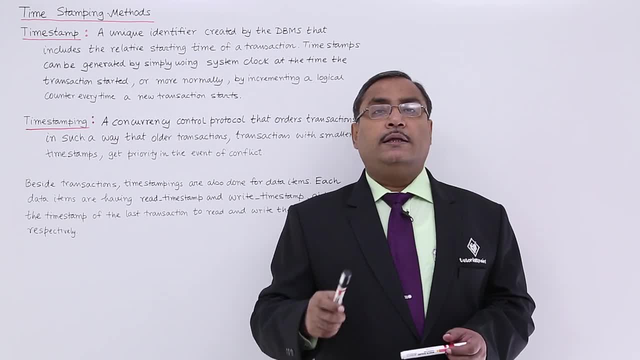 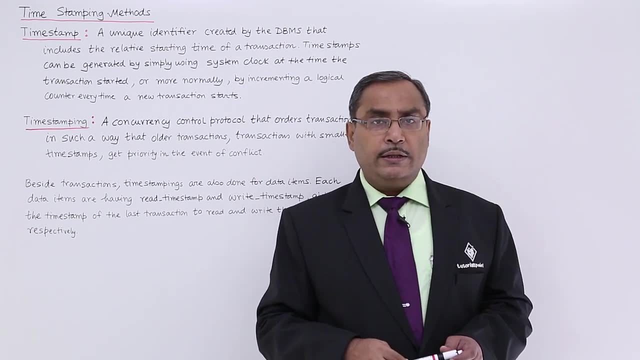 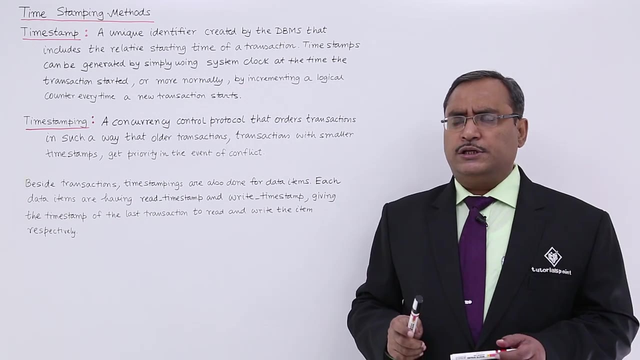 forward profit priority to the older transactions. then the transactions with the lesser timestamp value will get the priority higher compared to the transaction having the higher timestamp values. So this is the timestamping, So not only on the transactions. also we will be putting this. 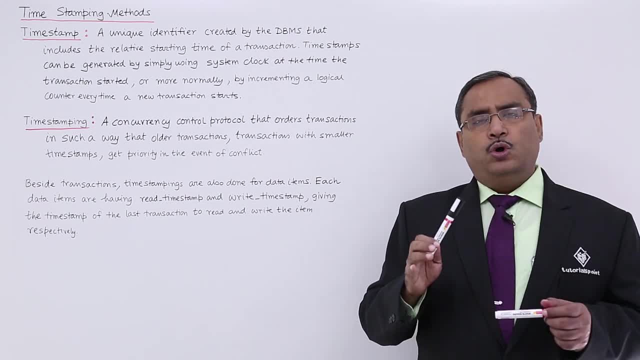 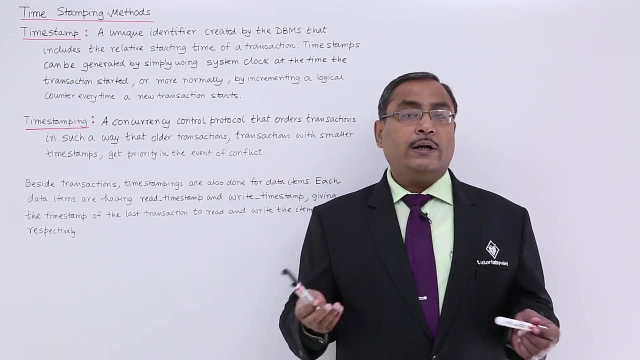 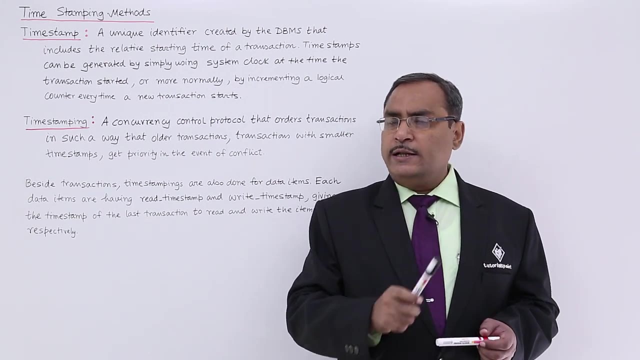 timestamping on the data items. So, on the data items, we will be having two timestamp: One is a read timestamp, another one is a write timestamp. What is the meaning of this read timestamp and write timestamp? The last transaction which has read this particular data item?